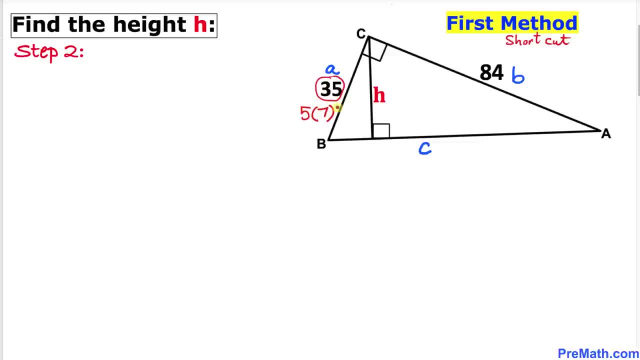 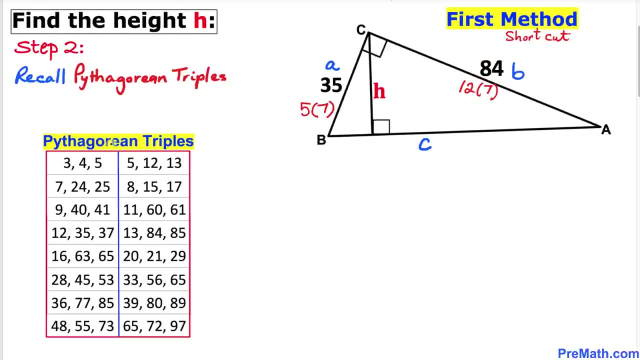 5 times 7, and likewise this 84 could be written as 12 times 7, and likewise this 84 could be written as 12 times 7, and likewise this 84 could be written as 12 times 7. and now let's recall Pythagorean triplets. and here are our Pythagorean triplets. Over here we can see: 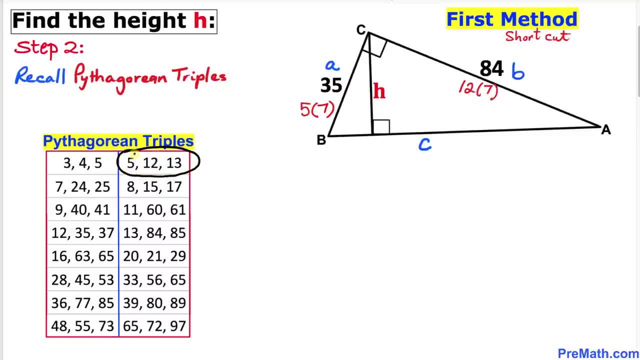 that this is going to work for us. We got 5, 12 and 13, and here we can see: we got 5, here we got 12, so that means this number is going to be 13 and since all these numbers are being multiplied by, 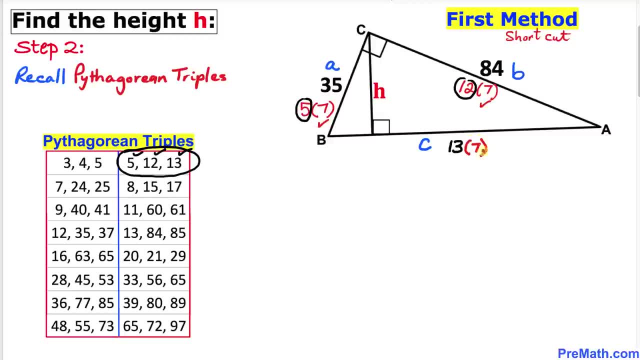 7. so I'm going to multiply them by 7, and I'm going to multiply them by 7, and I'm going to multiply by 7 as well. Therefore, our this side length c is going to be 13 times 7 is going to be 91. so thus, 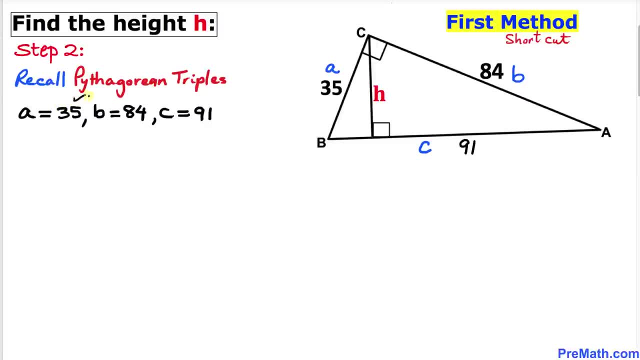 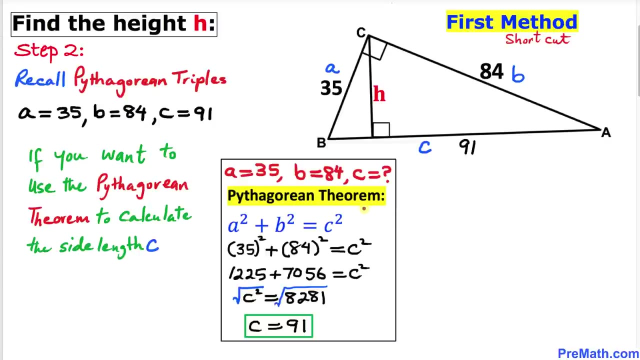 our side lengths a, b and c turns out to be 35, 84 and 91, and if you want to use the Pythagorean theorem instead to calculate this side length c- and here it is as a courtesy, I use the Pythagorean theorem. 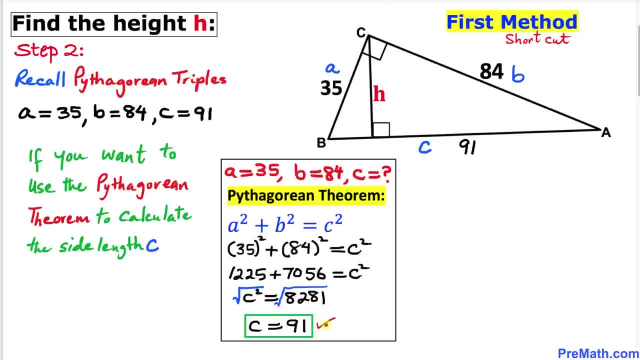 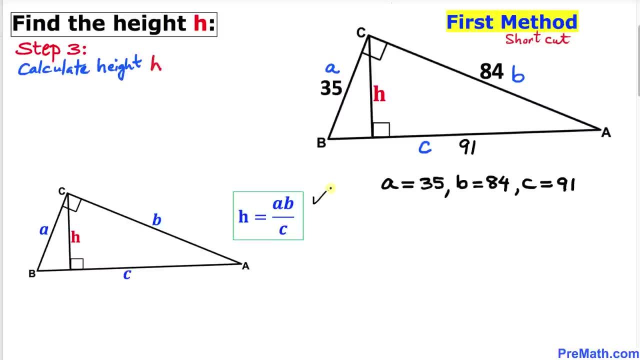 And I figured out the side length c, which is 91 as well. Now let's go ahead and calculate the height h, and here's the formula that we will be using to calculate h. h equals to a times b divided by c, where c is the hypotenuse of this triangle abc. So let's go ahead and apply the formula h equal to 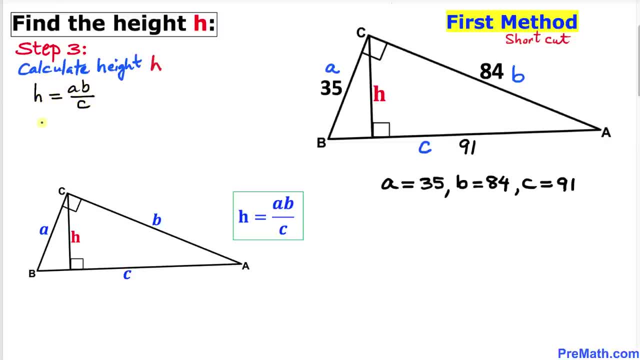 a times b divided by c- Let's fill in the blanks: h equal to a, in our case, is 35, b is 84, divided by c is 91, and if we calculate this one, so h is going to be approximately equal to 32.31 units. Thus our height h turns out to be: 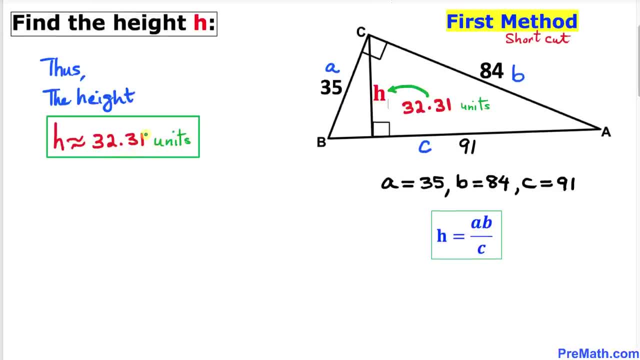 approximately equal to 32.31 units. And now let me share with you a formula for the height h. So let's go ahead and apply the formula and in this method, I will show you how we have come up with this formula. And now let's recall the. 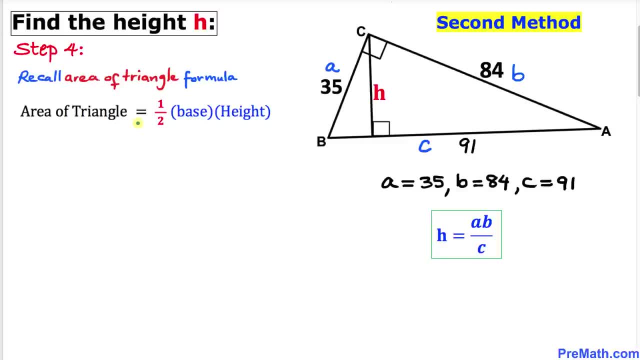 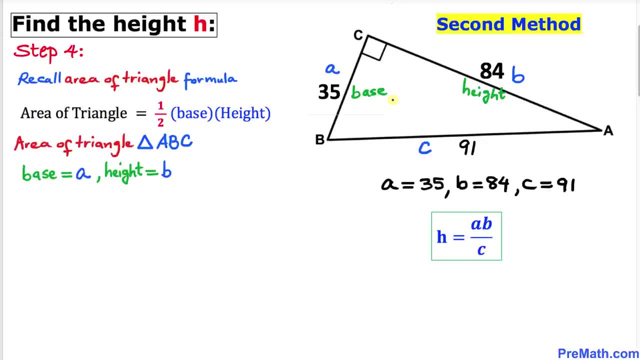 area of a triangle. formula: Area of a triangle is always equal to a half times base times height. So the area of this triangle, abc, is going to be when our base is a and height is b. We are going to apply this formula: Area is going to be height base a times b divided by two. Now let me go ahead and call. 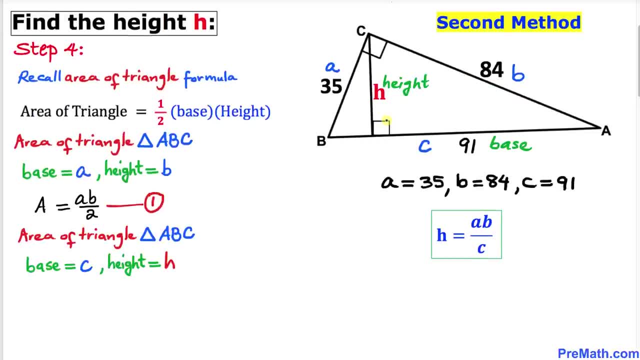 this equation as equation number one. Now let's go ahead and calculate the area of this triangle abc when our base is c, as you can see, and our height is h. Let's go ahead and apply this formula. So area of this triangle abc is equal to a times b, divided by 2.. 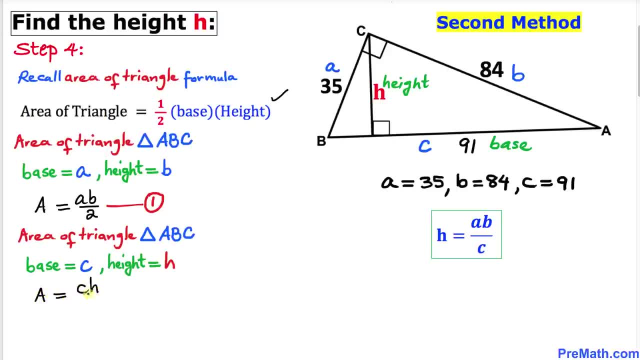 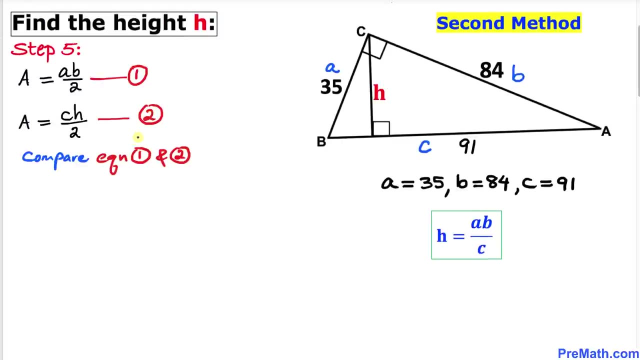 c is going to be c times h, divided by 2. and now let me go ahead and call this equation as number 2, and in this next step, we have got these two equations. now let's go ahead and compare these two equations. since the left hand side is same, so we can equate the right hand side as well. 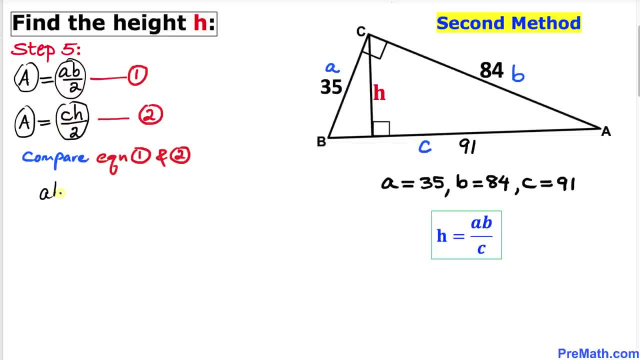 so I can write: a times b divided by 2 equal to c times h divided by 2. let's go ahead and remove the fraction by multiplying by 2 on both sides. so this 2 and 2 is gone. this 2 and 2 is gone. 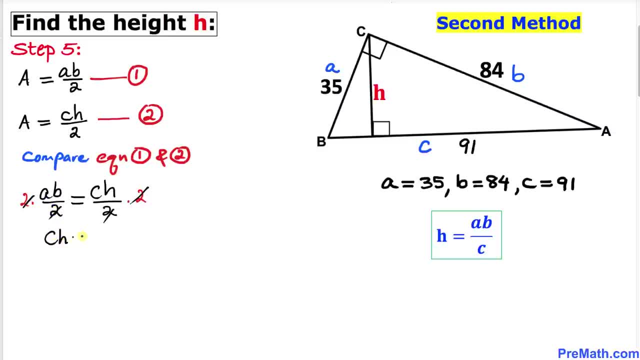 so we ended up with c times h equal to a times b. let's divide both sides. so we ended up with c times h equal to a times b. let's divide both sides by c, so c and c is gone. so h value turns out to be a times b divided by c, and that is our proof. 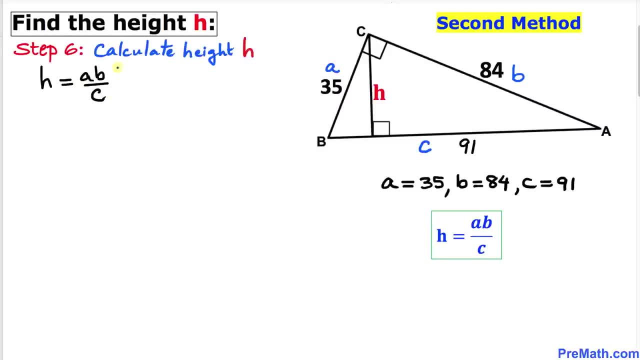 for this formula, and here's our final step. let's go ahead and calculate the height h, and we will be using this formula. so height is going to be: a, in our case is 35, b is 84. divided by c is 91. if we calculate and simplify, our h value is approximately equal to 32.31 plus our height.